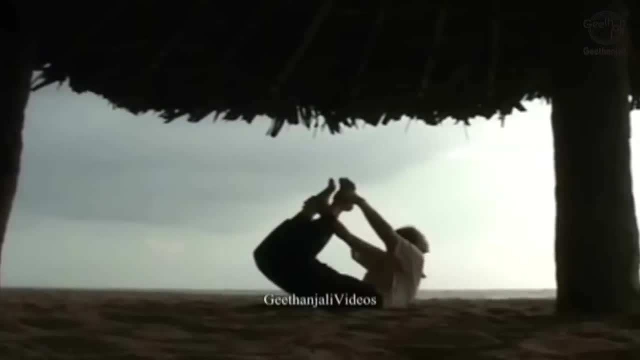 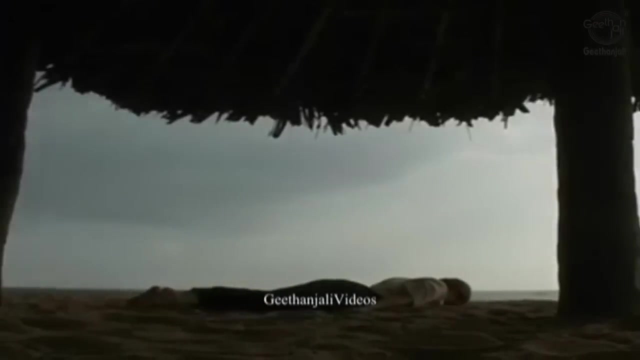 Do not do this posture if you suffer from any diseases of the liver or kidneys, as the intense pressure may be too much for the weak organs. Keep it straight until every train of thought and effort to the stomach is absorbed. Keep your legs at a distance and bear in mind your body is equipped with a constant weight of strength. 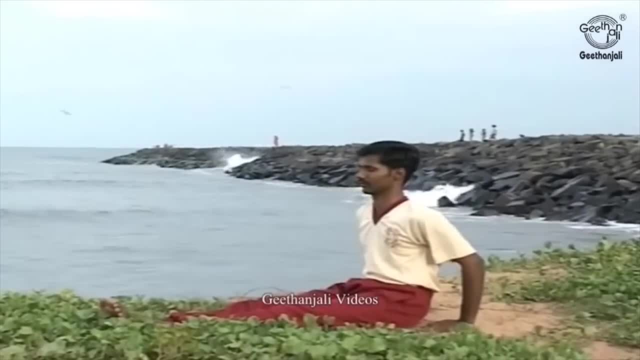 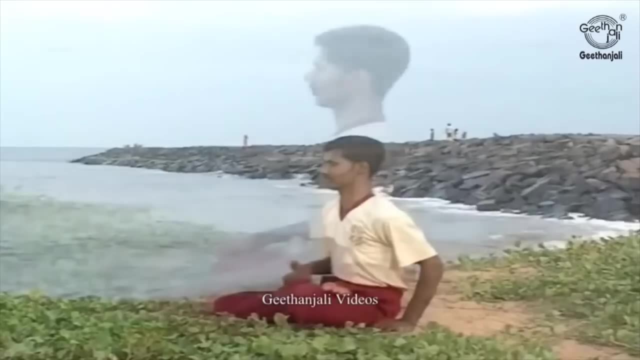 Sit straight with your legs stretched out in front. Fold up your legs and perform the Padmasana. Bend your elbows and relax backwards until your legs are straight and your body is upright. Have your body fully relaxed and your lower body is in the correct place. 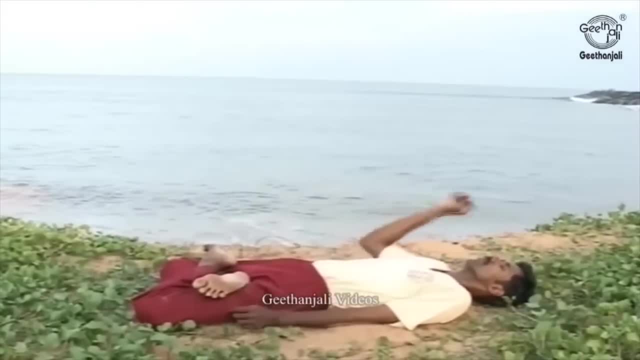 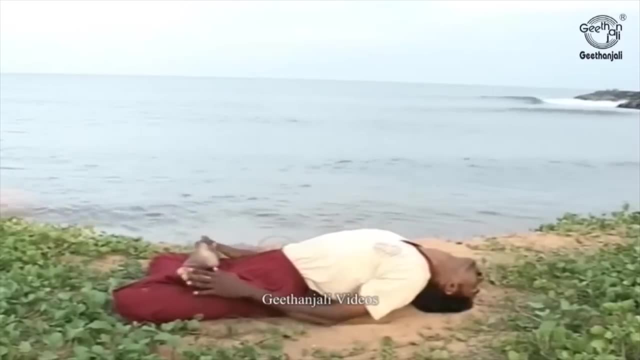 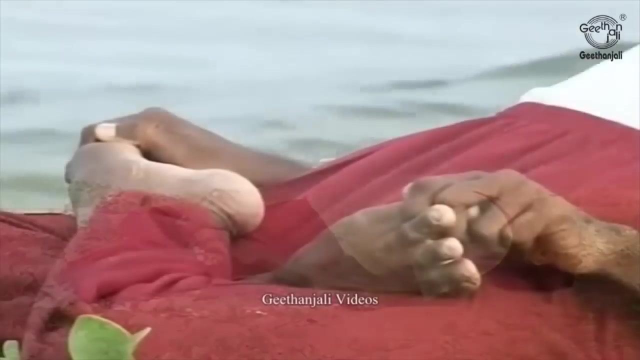 Hold the knees with your feet and do the Padmasana from the same place. your elbows are flat on the ground. Use your hands to lift the shoulders off the ground in an exaggerated back bend until your entire weight is balanced on the top of your head. If possible, catch, hold of your toes with your fingers and bring. 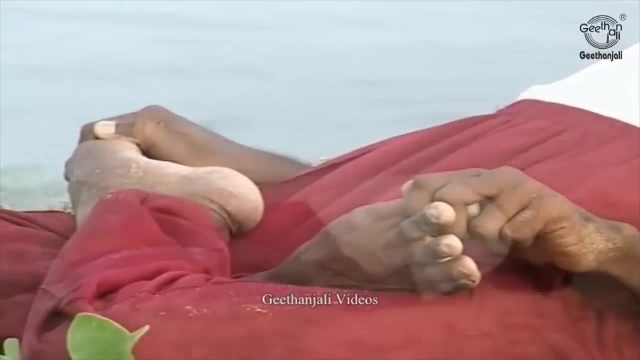 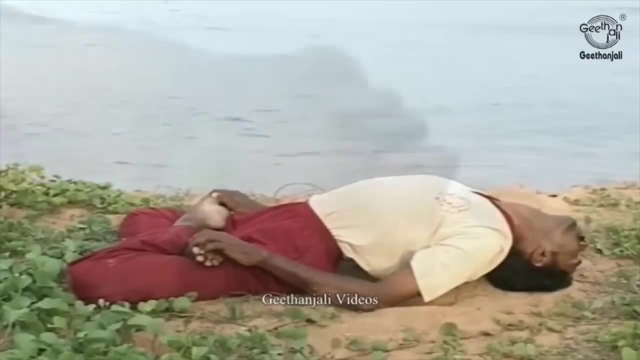 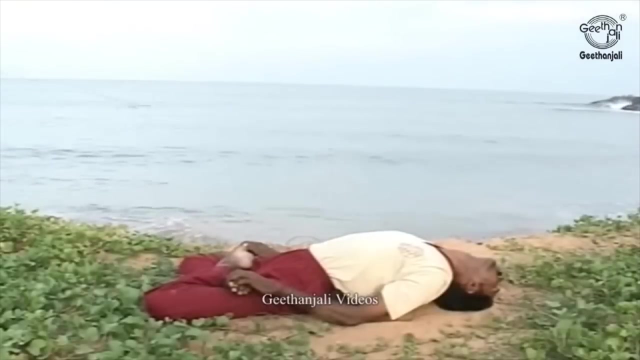 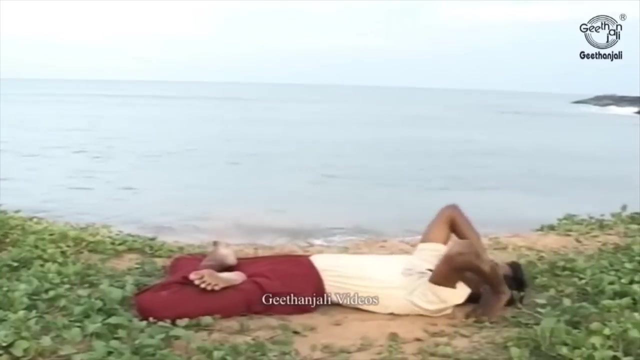 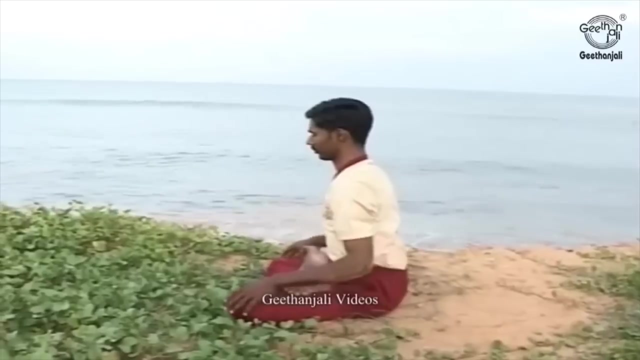 both your elbows down to the ground. Perform three to nine rounds of deep breathing in this position. When ready, return back to the Padmasana in a careful, step-by-step manner. Unlock your feet and stretch them forward into the Uttanasana and then. 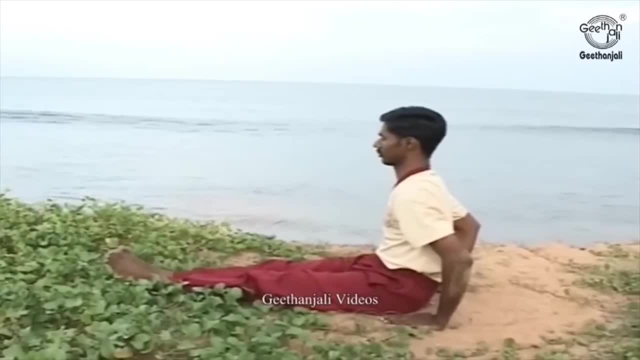 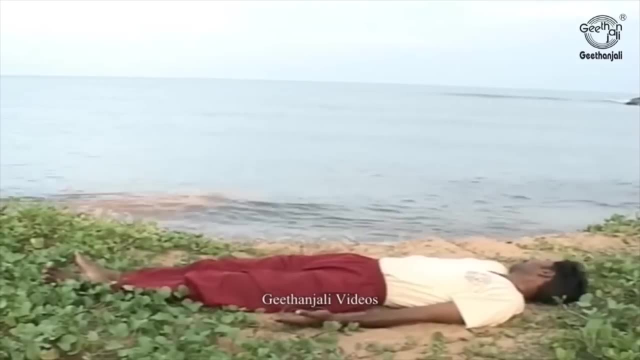 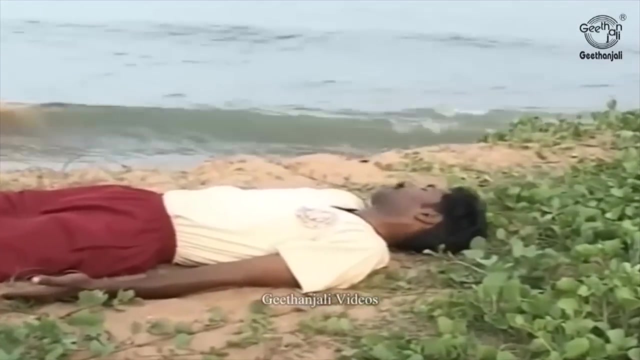 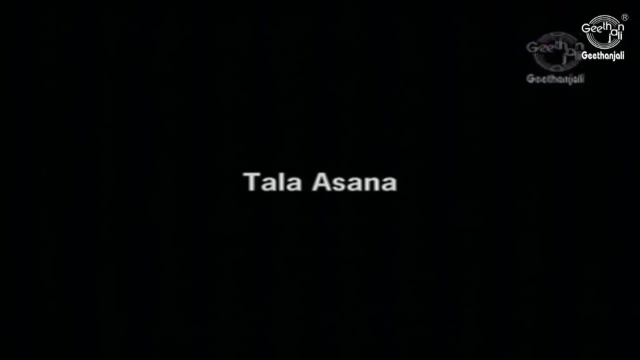 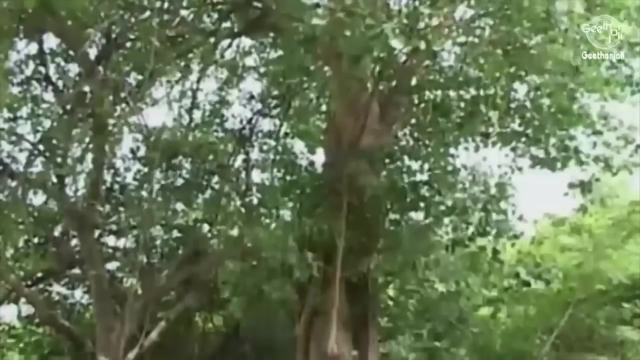 slowly return to the supine. Shavasana A. A couple of rounds of head rolling from side to side in Shavasana can help release any pent-up tension in the neck that may occur after performing the fish posture. Talasana: Take up a comfortable and stable Samasthiti Asana. 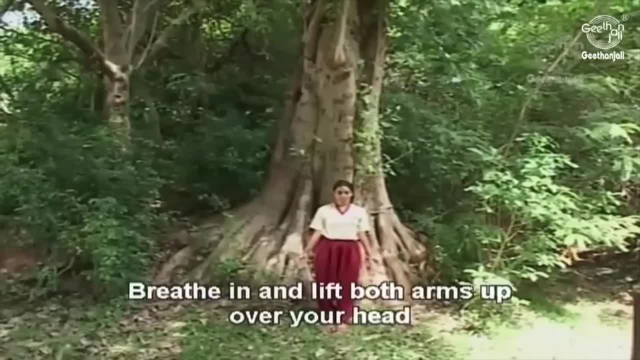 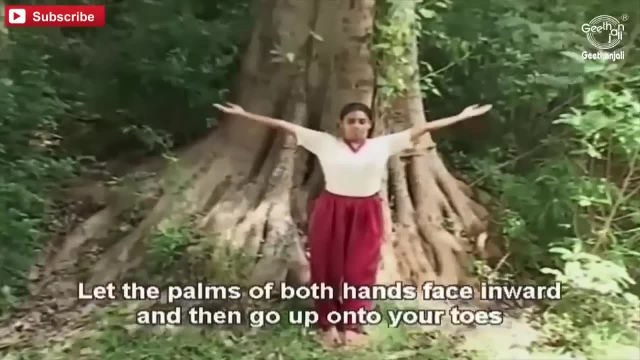 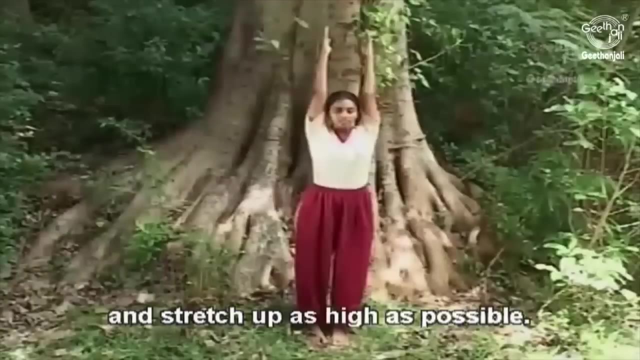 Breathe in and lift both arms up over your head until they are parallel to each other. Let the palms of both hands face inward and then go up onto your toes and stretch up as high as possible. Hold the breath and feel the healthy stretch along your whole body, from toes to fingertips. 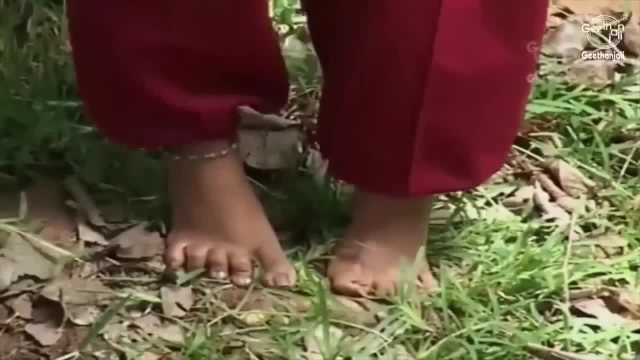 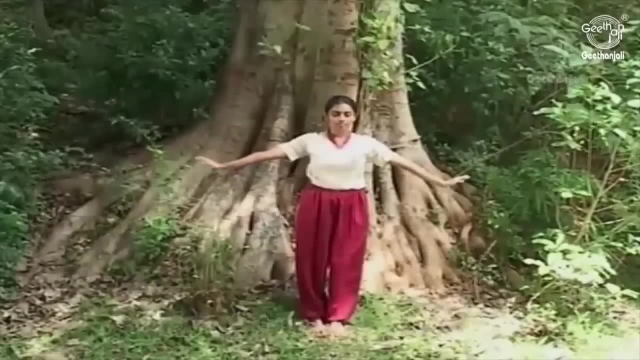 Breathe out and relax your arms back to your sides when you are ready to start, Hold the breath and feel the muscles in your hands. Breathe out and relax your arms back to your sides while coming back to the flat foot posture. 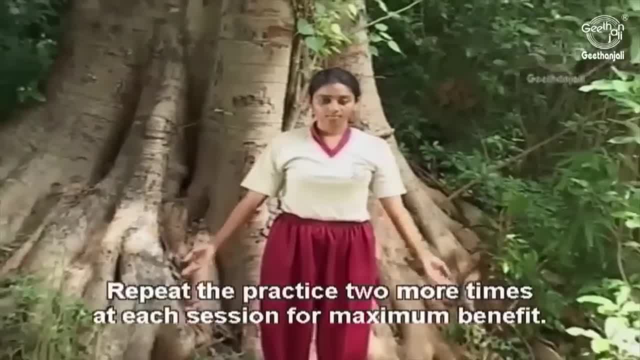 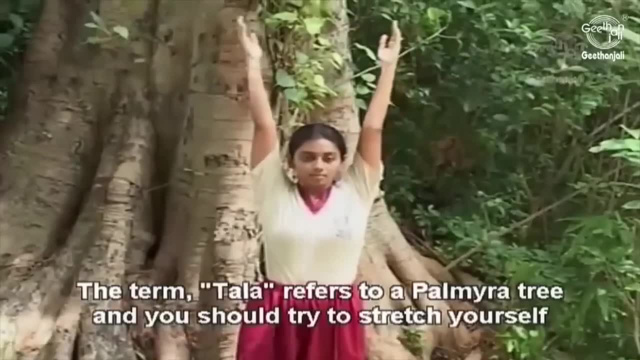 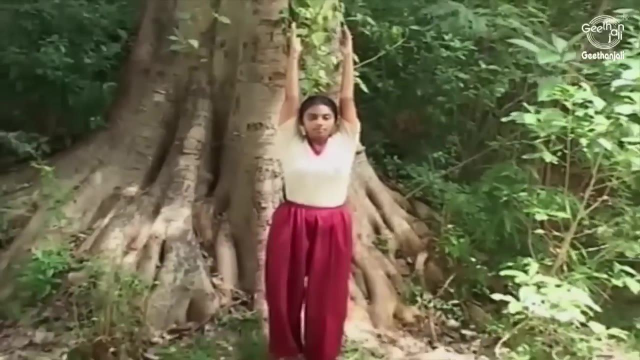 Repeat the practice two more times at each session for maximum benefit. The term Tala refers to a Palmyra tree, and you should try to stretch yourself as tall as that tree while performing this practice. With practice, the posture can be held for a longer time. 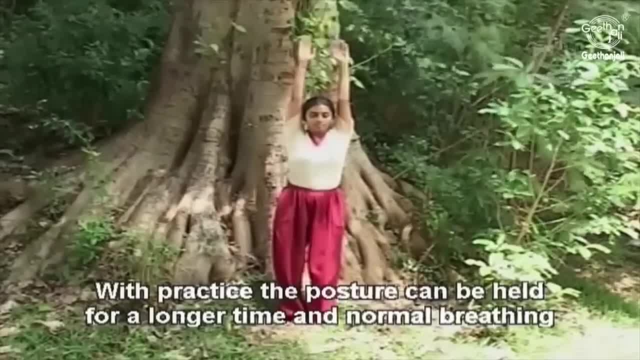 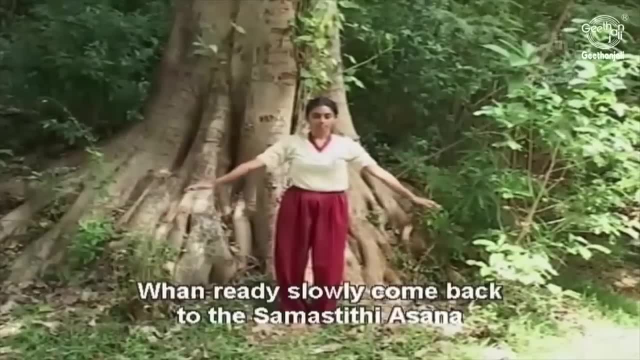 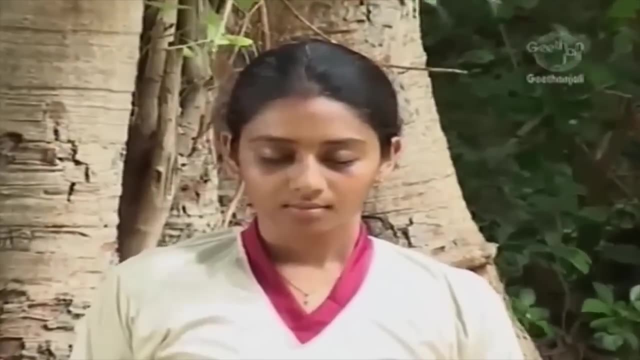 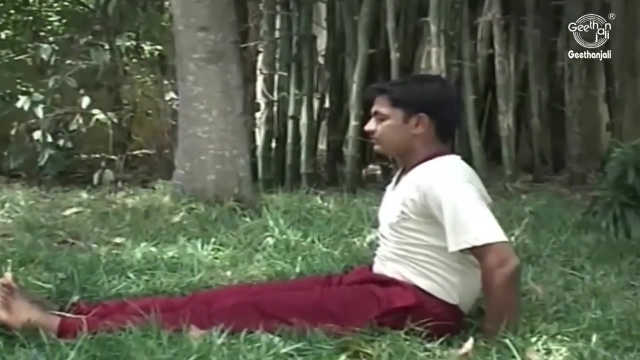 A normal breathing, done while holding the palm of your hand, holding the posture for 30 to 45 seconds. When ready, slowly come back to the Samstiti Asana and relax with a few rounds of deep breathing. Purvottanasana In Uttanasana: place the hands behind the back. 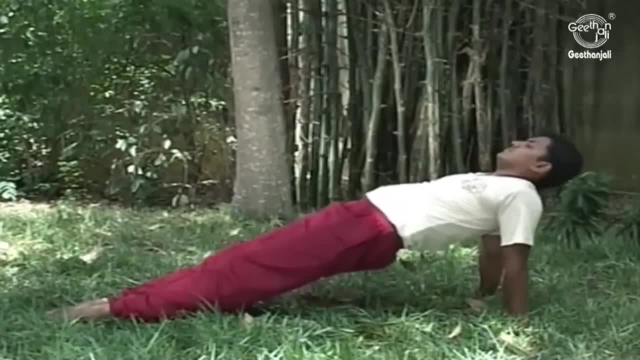 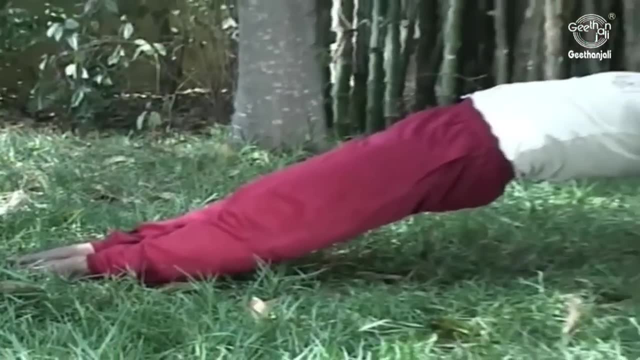 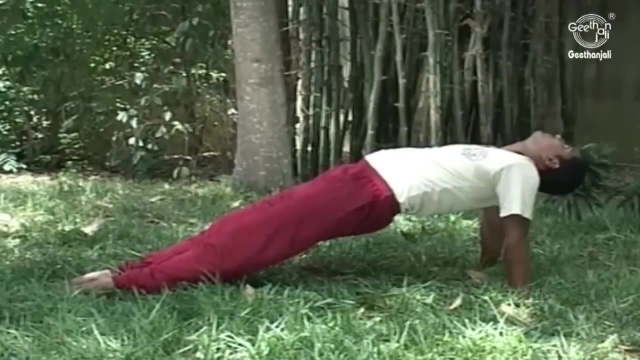 with the palms on the ground On an in-breath. lift the body so that the entire body is arched, from the feet that are flat on the ground to the head that is loosely dangling between the shoulders. The fingers must point towards the back. 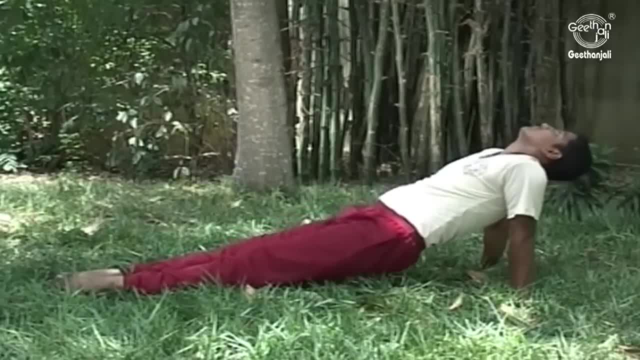 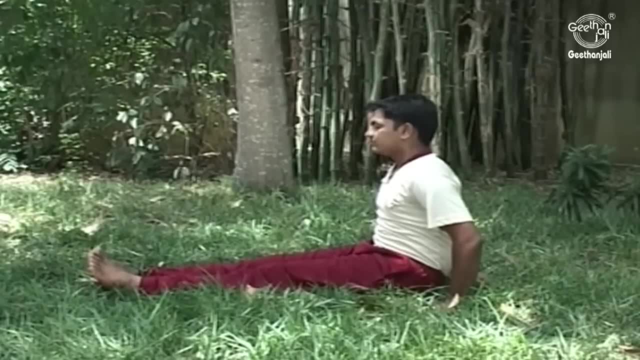 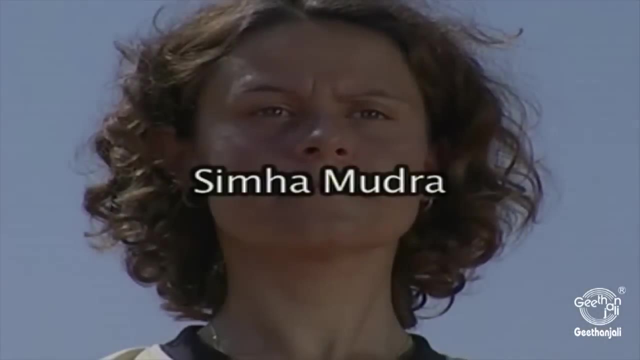 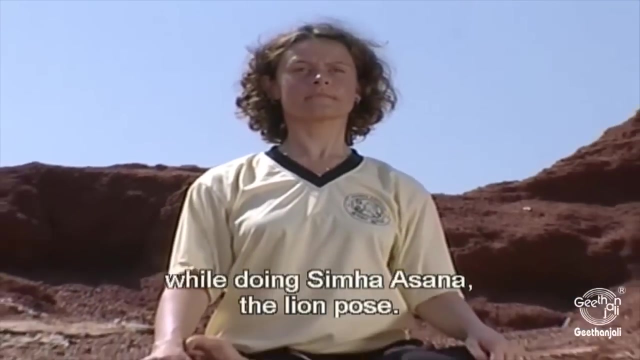 Release the pose on the out-breath and relax in Uttanasana. This is a good complementary pose to both Paschimottanasana and Halasana. Simhamudra, The lion gesture- has a special arrangement of the jaw and tongue while doing Simhasana. 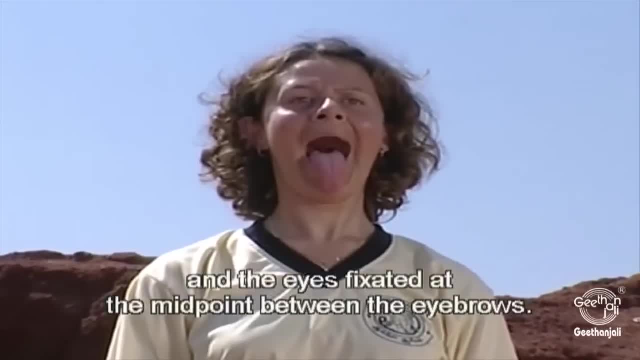 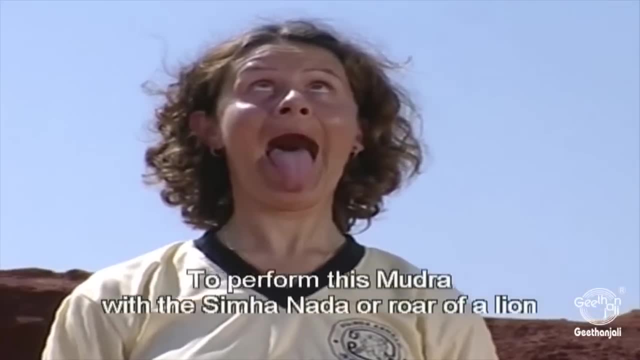 The tongue is extended as far as possible and the eyes fixated at that mid-point between the eyebrows To perform Simhasana with the Simha Natha. the eyes must be fixed in the middle of the eyes. The eyes must be fixed in the middle of the eyes. 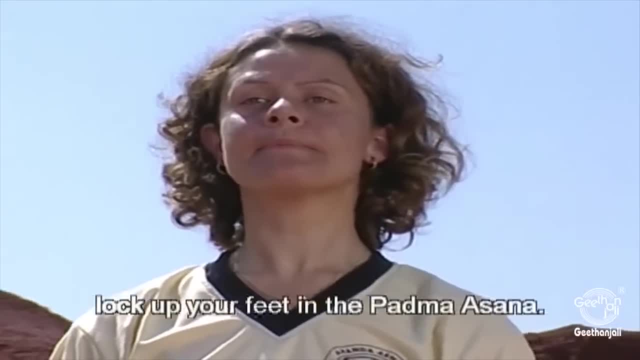 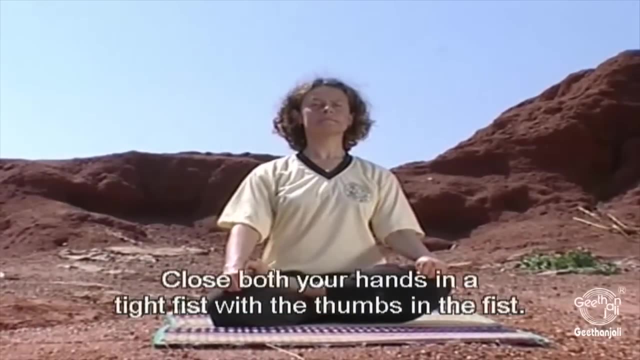 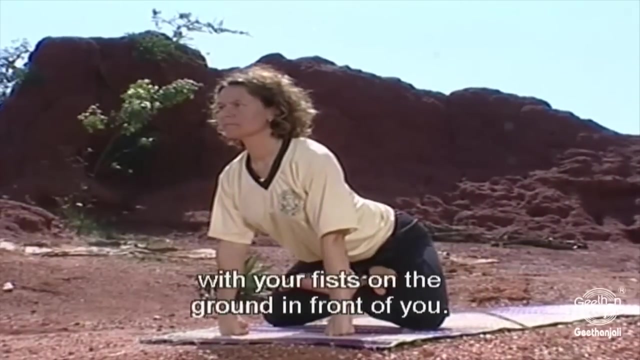 or roar of a lion. lock up your feet in the Padmasana. Close both your hands in a tight fist, with the thumbs in the middle of the fist. Come onto your knees and balance with your fists on the ground in front of you. Take in a deep breath while lowering your.